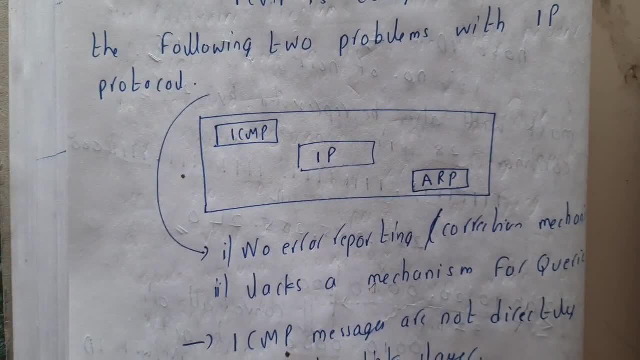 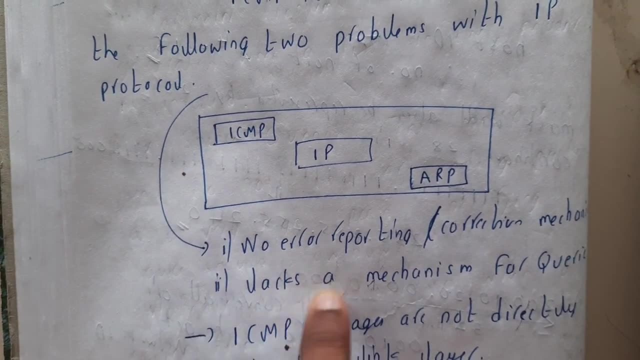 in IP So you cannot say that there is an error or there is a how to resolve it. like that you cannot send any kind of messages. So basically, this is nothing but messages, guys okay, and lacks a mechanism for queries. So basically, to ask some kind of questions or queries, you cannot do it in. 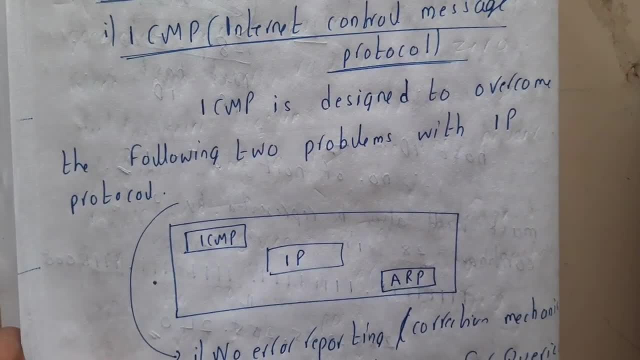 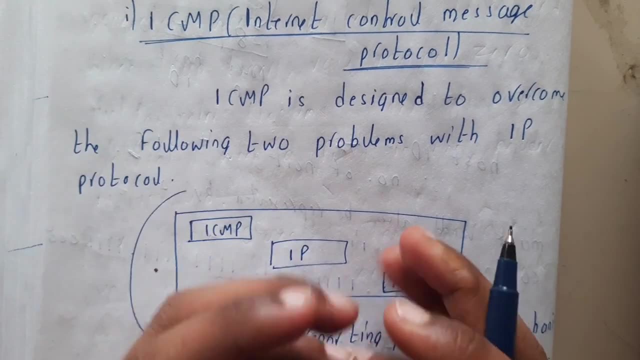 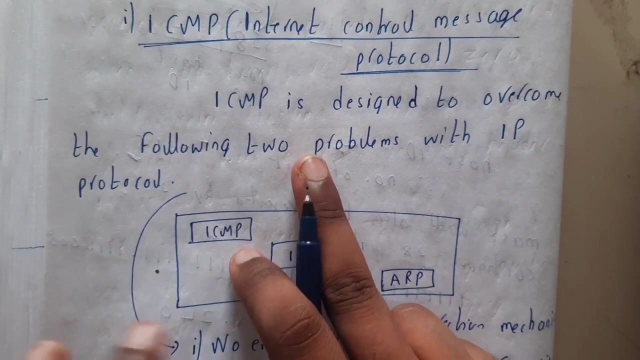 using IP. okay, So this ICMP is inside IP. you can assume in that way, guys, because it is wrapped inside IP. okay, So inside IP you will be having ICMP. you can assume in that way also. okay, So let us go through. So that will be having a clear idea. ICMP is designed to overcome the following two problems: 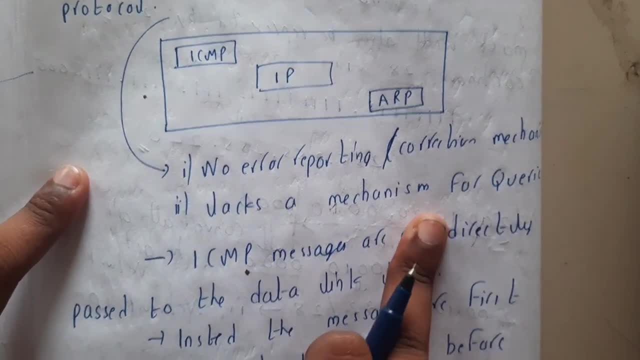 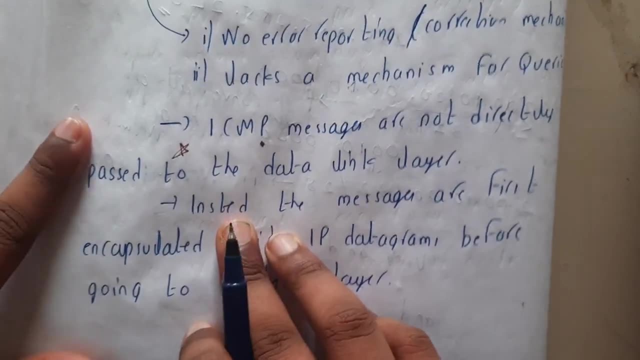 No error reporting or correction mechanism lacks a mechanism for queries. So ICMP messages are not directly passed to the data link layer. Remember that it cannot be sent directly. Instead, the messages are first encapsulated inside the IP datagram. that's what I told you before going to. 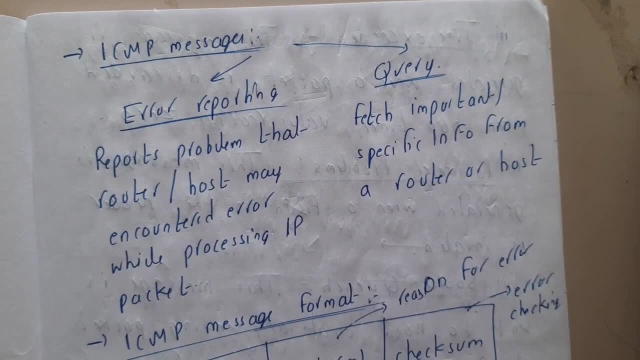 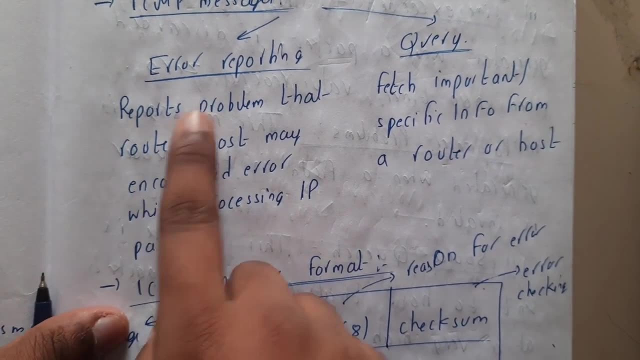 the lower layer. So IP protocol packets and those things are really mandatory guys. okay, So ICMP can send two kinds of messages. So ICMP messages are not directly passed to the data link layer, So it can send two kinds of messages. That is nothing but error reporting. So reports problems that 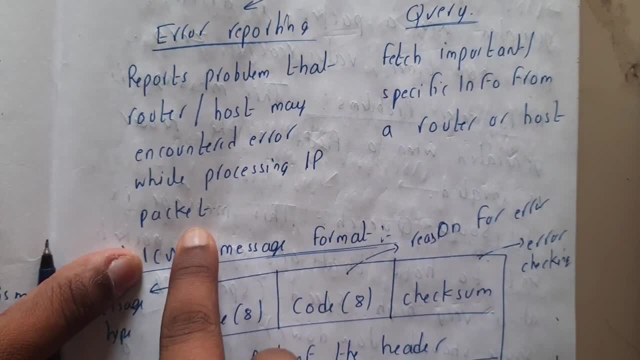 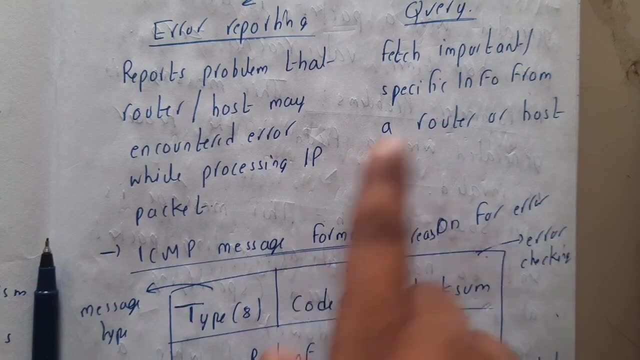 routers, hosts may encounter error while processing the IP. So if they face any kind of issues, we'll be storing the message and we'll be resending it. That is nothing but error reporting. Similarly, query fetch important and specific info from the router or host, So to get a specific information. 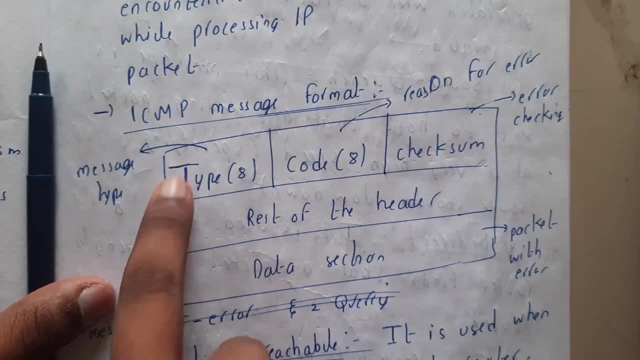 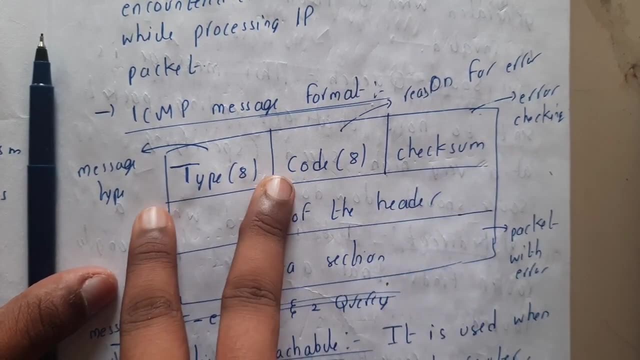 we can do this operation also. So the ICMP packet will be in this way. okay. So again, this also is a 32 bit. I think so, guys, I'm not sure about it. Okay, 32 bits, 8 bit type and 8 bit code and 16 bit of sum. okay, Similarly, the type will be saying that: what is the? 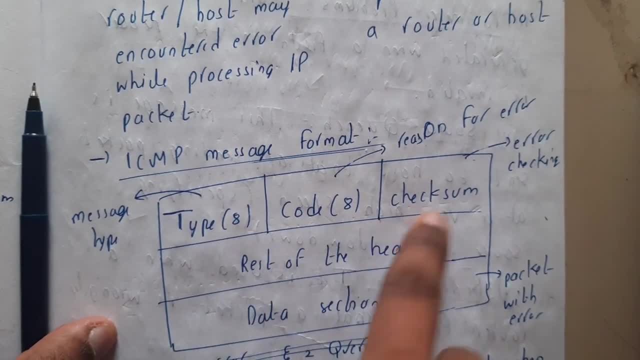 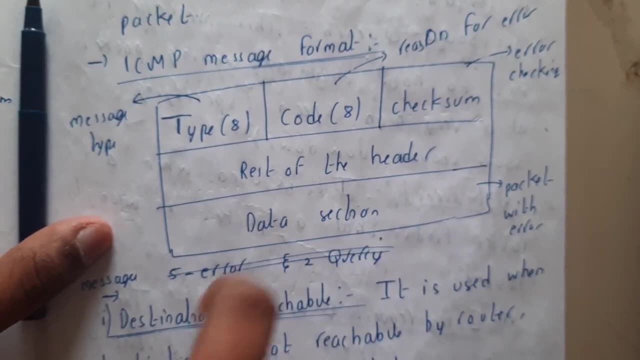 message type Code will be saying the reason, like what is the issue, and checksum will be used for checking the error and the rest of the header will be the same. and data session. Data session is nothing but packet with the error, So whatever is there, that will be shown here. okay, So now let us. 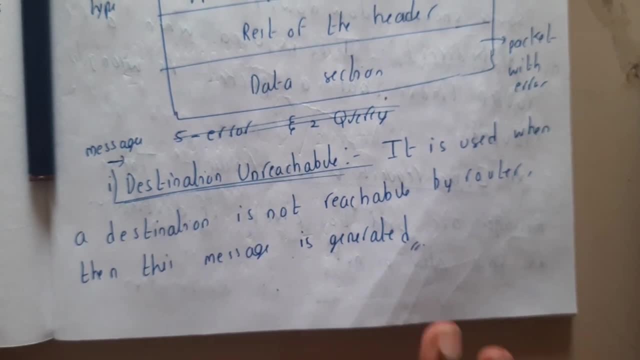 go through some messages, guys. What are the messages? I'm saying messages, messages, right. So now let us go through messages. So, destination unreachable. So it clearly says that the destination is not available or unreachable. So it clearly says that the destination is not available or unreachable. So 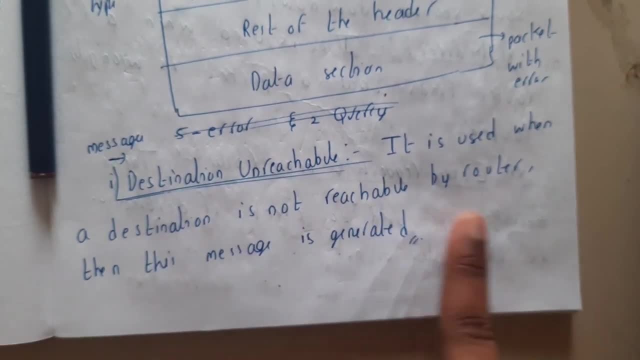 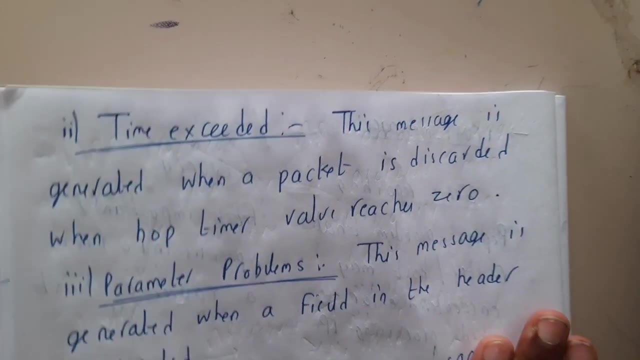 we cannot reach that router, So it is used when the destination is not reachable by the router. Then this message is generated backwards, So this will be received by the host. Okay, time exceeded. So these messages are really from the name. only you can identify, guys. 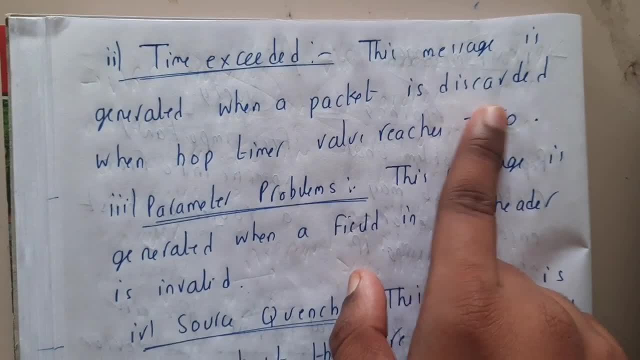 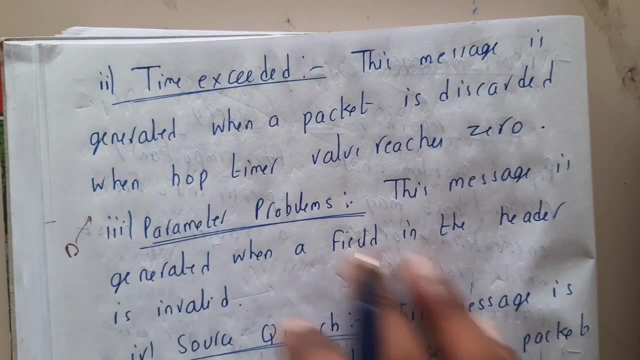 Time exceeded. This message is generated when a packet is discarded, when hop timer value reached to zero. So basically, if you sent a packet to a particular IP and you'll be thinking, you'll be just enjoying your time, right? So you'll be thinking that it will be reached sometime. 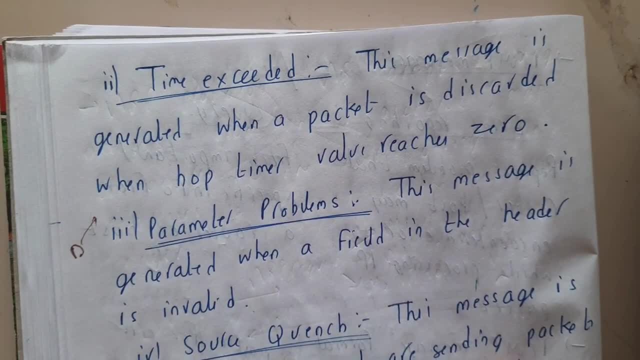 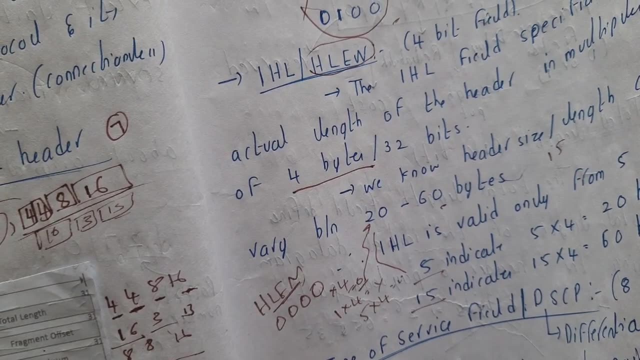 So, but it will be having a time time, guys. That is nothing but a time of death, or it will be. just give me a second. I'll be just seeing the name, so that you'll not be having any type of confusion. Time to leave, guys. 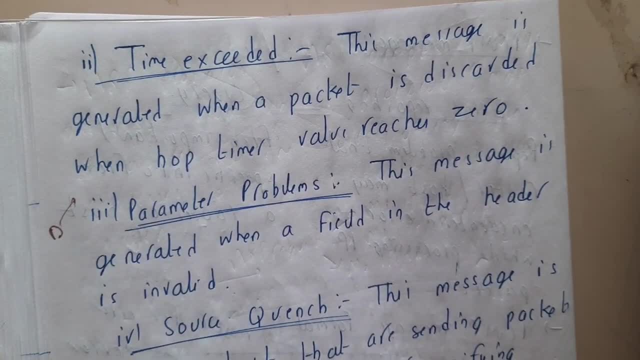 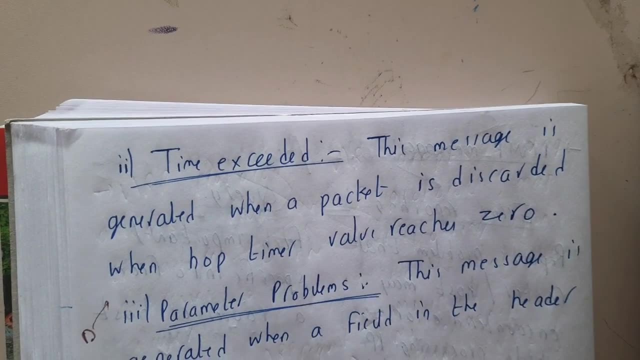 T-O-L. That is nothing but time to leave, Okay. T-T-L. sorry, T-T-L. Time to leave, Okay. So once that time has been exceeded, it will die or it will be lost directly. It will be discarded. So for those kind of packets, 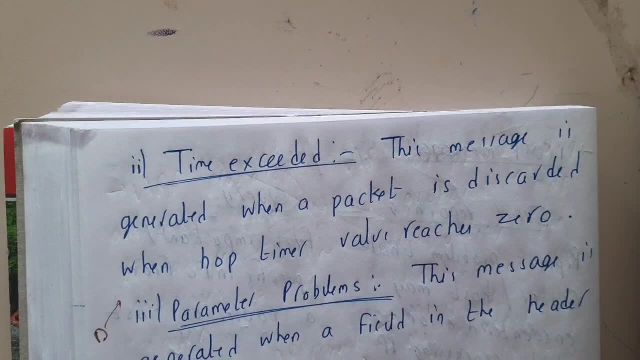 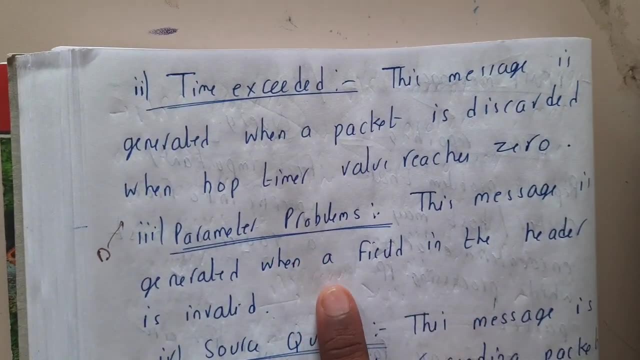 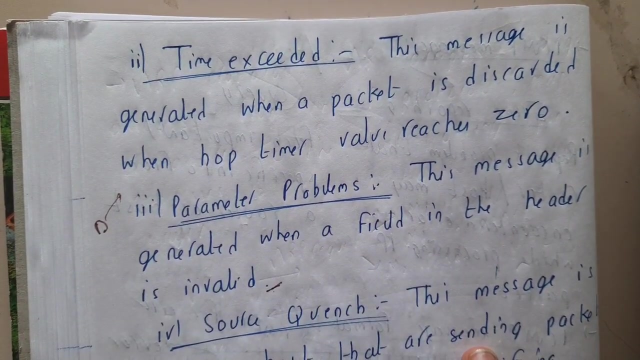 we don't know whether they are reached or not. So this time extended will be saying that whether if it is time has been exceeded, It will be sending a packet in a reverse way. Okay, Similarly, parameter problems. So this message is generated when the field in the header is invalid, So when there is any kind of issues like corrupted. 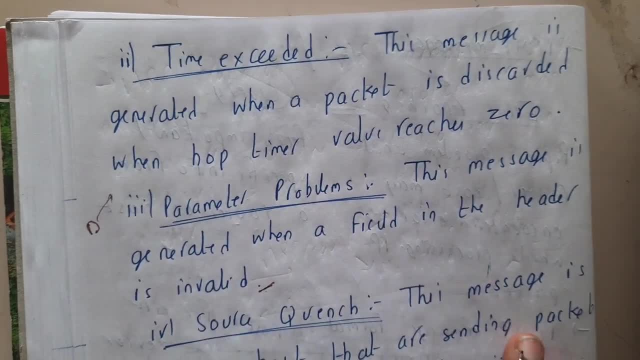 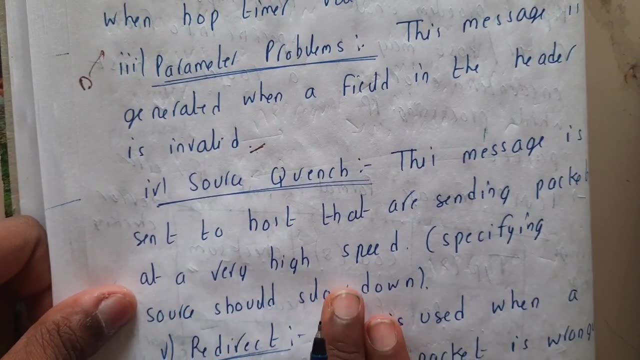 corrupted files or anything, then we'll be getting this as a result. Okay, Similarly, source quench. So this message is a sent to the host that are sending the packets at a very high speed, specifying source to slow down. So when there is a faster sending of data, then we want to return the 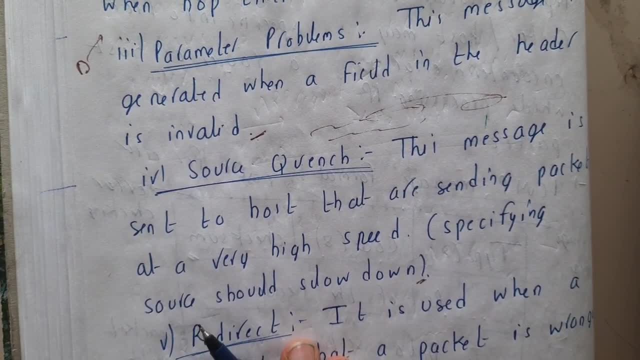 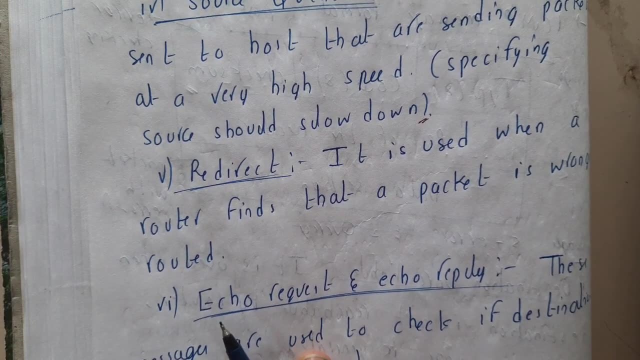 packets right. So he will be sending a packet saying that please slow down, slow down, and he will be slowing down. So that is nothing. but this is source and similarly redirect. So from the name itself you can say So. it is used when a router finds that a packet is going in the wrong route. 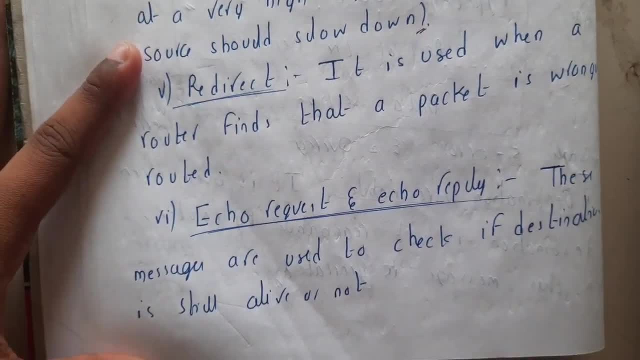 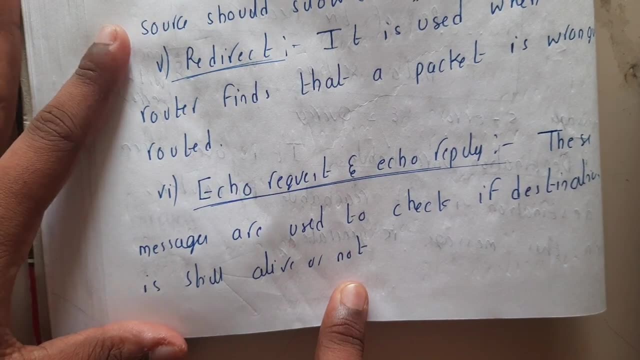 Okay, so it should be redirected to the correct path: Echo request and echo reply. So these messages are used to check if destination is still alive or not. So, basically, this is nothing but echo request. So you will be requesting. the server will be requesting.